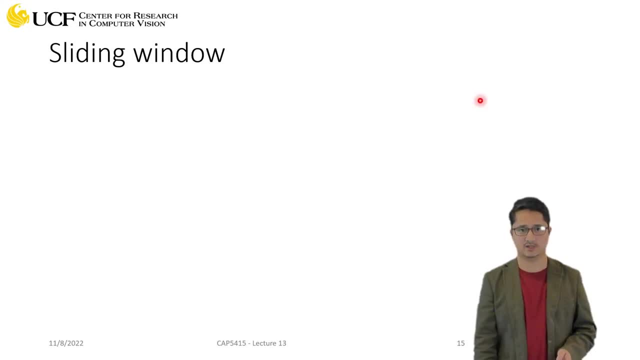 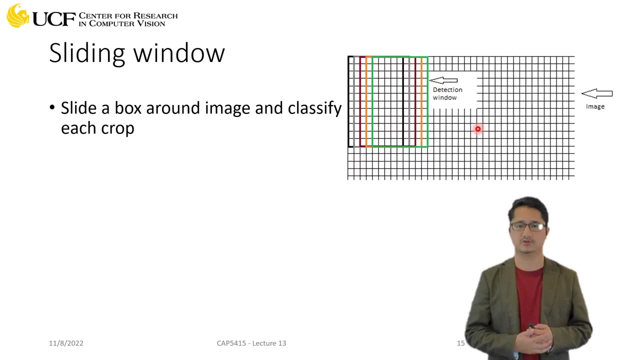 you have. you have required the sliding window approach and today as well, you will see like how this is going to be useful for object detection. okay, so a simple solution could be: if this is your input image and you want to detect like some object in this image, you can take a window. okay, a bounding box and wherever you are placing. 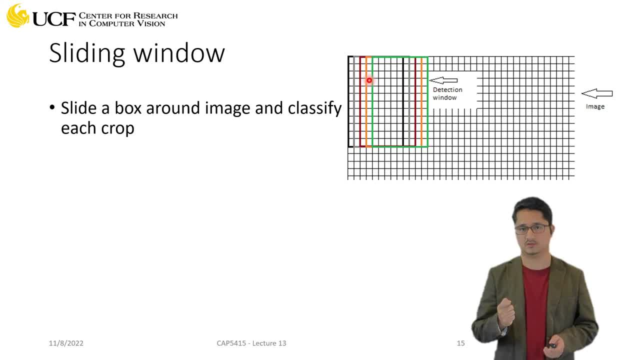 that window you can try to detect your object, and you know how to do that. you can just use filtering, or you can use like any other algorithm as well, but filtering is just one, and then you can just keep sliding that throughout your input image. okay, so all the possible locations where you can place. 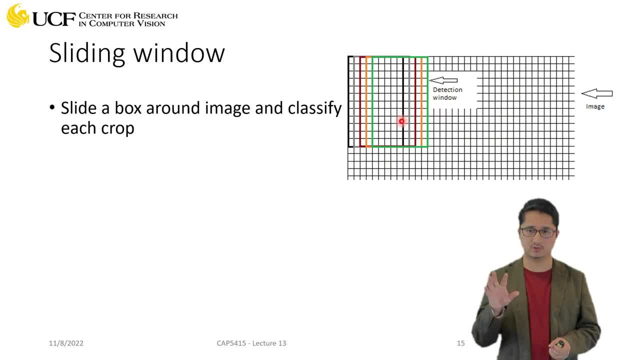 it and then, at whichever location gives you like the highest probability of detection, you can say: okay, this object is present in that particular location. so that's, that's like a very, very simple, crude algorithm, uh, which which can be used and, of course, like there are a lot of, lot of interesting. 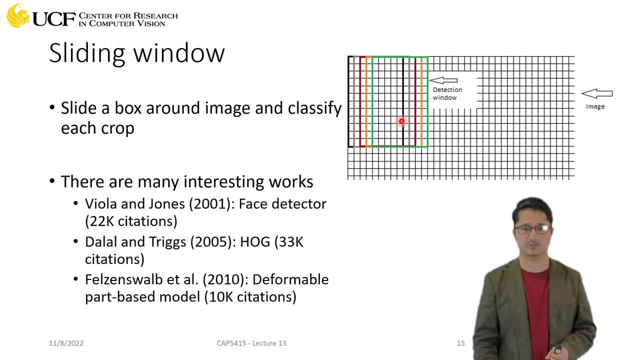 works out there which are actually using, uh, the sliding window approach, not just for person detection, but face detection as well. right and HOG, as i said, like it is also using sliding window and there are like a lot of other algorithms. just just to mention these three, but it's, it's a lot, uh, i think i used used a lot in. 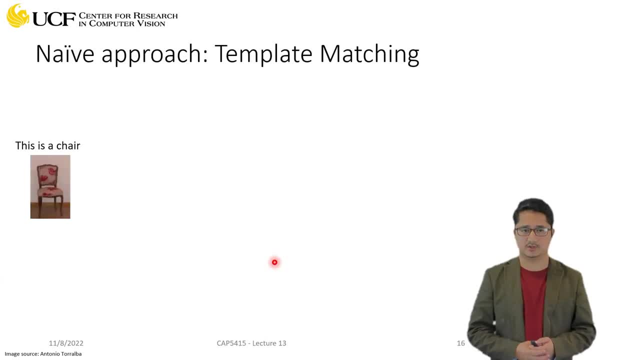 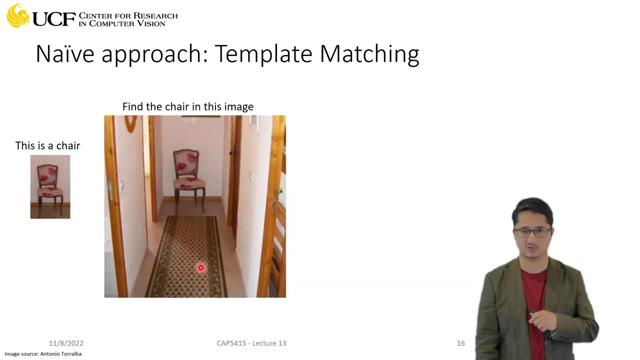 many, many other algorithms. okay, so let's see how we can do object detection. um, and again, this we have seen, but not from detection point of view, from classification point of view. but if you think about this, this is actually solving detection for you. so this is your chair. 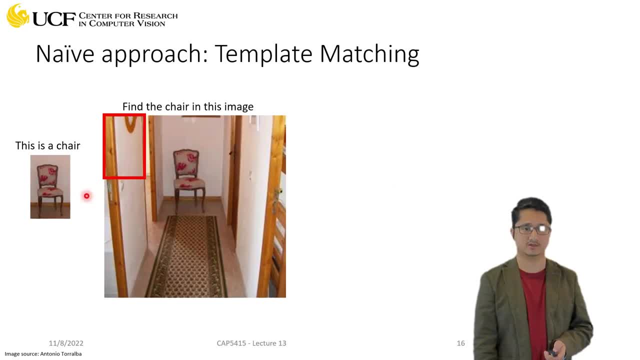 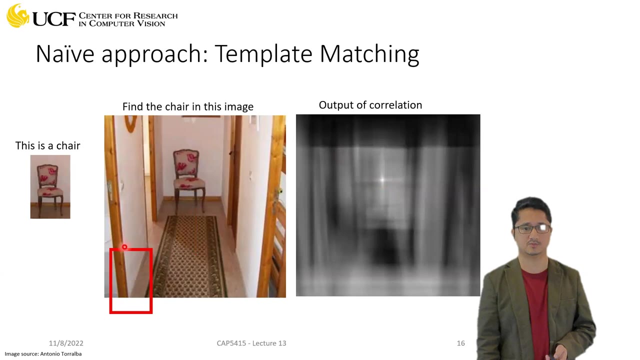 template. this is your original image and you can just try to match this template at all the possible locations in your image. okay, earlier we saw we can use that for classification, but now we know that this position is actually highly active. so we just put this morning box over here and we say that. 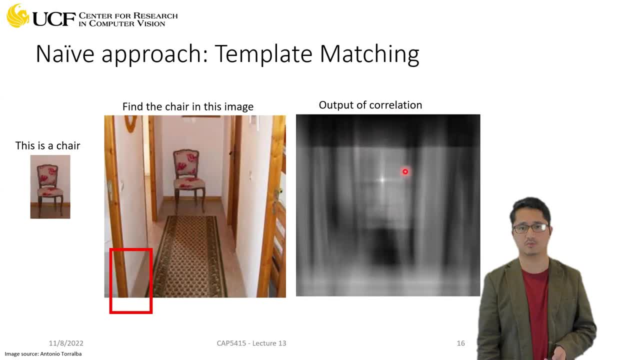 the chair is present at this particular location and it doesn't matter how big your image is or how small your chair is. if you have like a perfect matching template, you will be able to localize that okay. so this, this is like a very naive algorithm which can be used and, of course, we 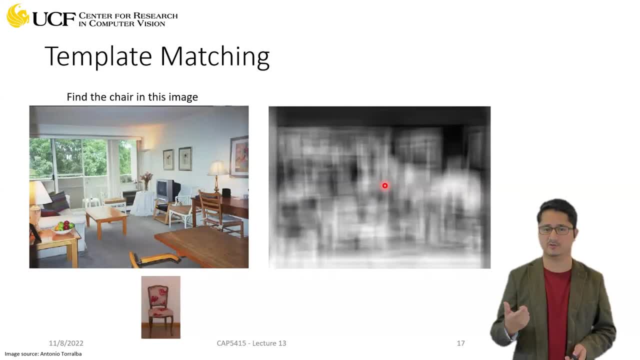 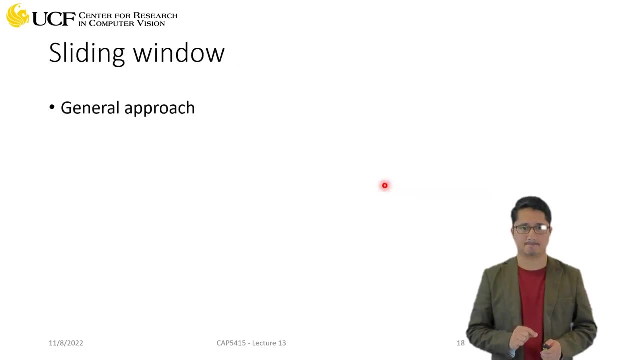 have seen, it will fail, like in in real world scenario, because template will change, there will even in the pose of chair, or there could be like color changes, lighting changes, but the, the intuition will not change and the basic approach won't change. okay, so let's try to understand how this can be done, like in a more realistic setting, so that 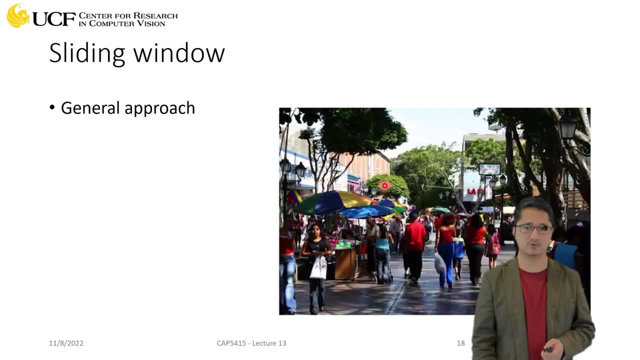 the algorithm actually works. it doesn't fail. okay, so the general approach will remain the same. you will have this uh input image where, let's say, we are interested in person detection and you can like, it's very crowded, so what you want to do is you want to detect all these uh individuals. 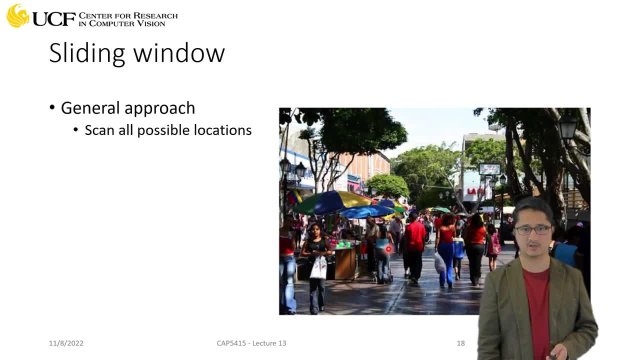 standing on the street or doing whatever they are they are doing. so what we do is we start with a bonding box and we, again, we do the same thing: we scan all the possible locations. okay, now, while doing that, we we don't use the template. now, coming back to, we have covered. 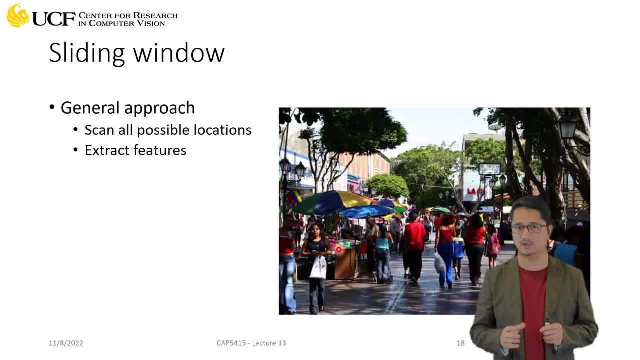 like a lot of algorithms for feature extraction. right, we covered classical approaches, we covered cnn based approaches. now we make use of those approaches and you will see, like, how features are, uh, very, very useful. so what you do from that location you extract feature no template matching. okay, for example, i told you could be like one set of features, uh, it could be sip features, it could. 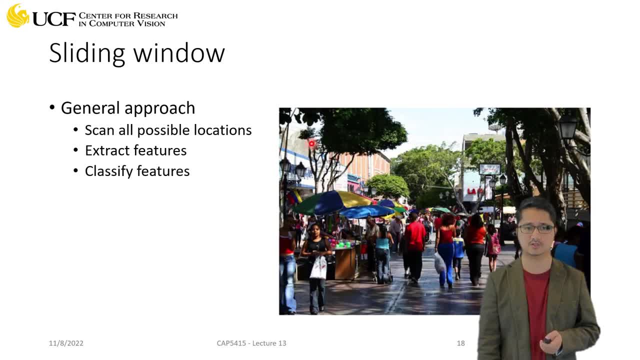 be cnn based features, it's up to you. a lot of options out there, then what we do is we try to classify those features. so instead of template matching, uh template matching, now we are doing classification, which is much more powerful than uh cnn based approaches, which is much more powerful. 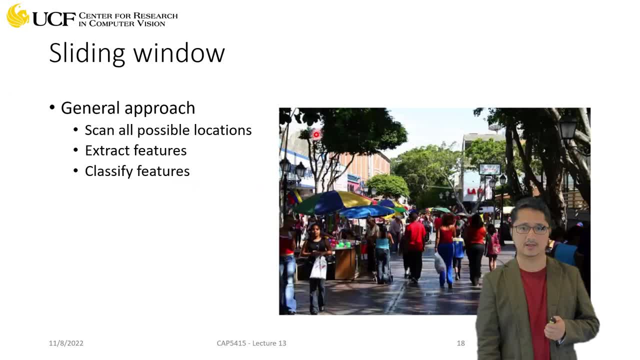 powerful than template matching. okay, so what will happen at each location where you are placing your bonding box? you are just trying to identify, using this classification algorithm, whether that object is present or not. so the algorithm remains the same, the one we discussed for the name approach. the only difference is we extract features and use those features for finding out whether object 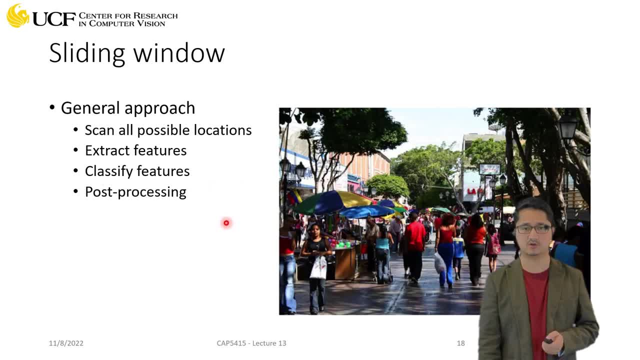 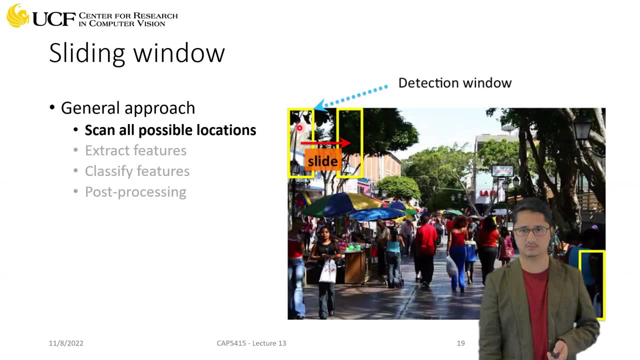 is present or not, and then some post processing is required, which i will talk about. that's really important, okay, so let's start so you scan all the features and you can see that the object is present, all the possible locations. let's say: this is your detection window, this slide and you inspect all. 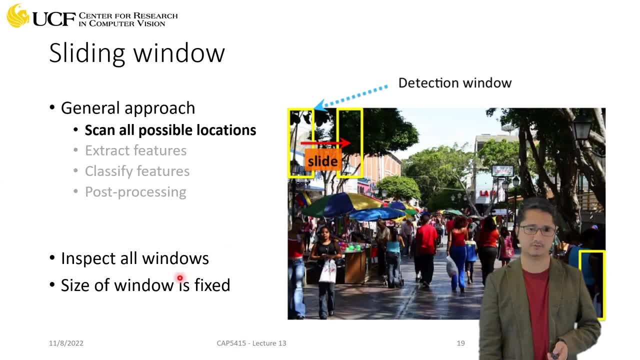 the- uh, all the windows. so in this case you can see like your window size is kind of fixed. now the issue is the person actually, which are the persons who are closer to the camera. you can see like you need a bigger bonding box and persons like far away from the camera, you need a very small bonding box. 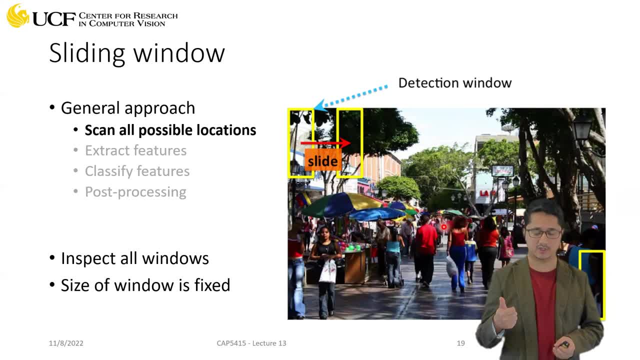 okay, so now you can understand, like, where i'm going with this. we were talking about sift features. so what did? what did we do there to solve this? we try at different scales, okay, so we created like that, uh, uh, that that's called the pyramid. right, we do exactly the same thing: we create pyramid and to create a pyramid, what we'll do is: 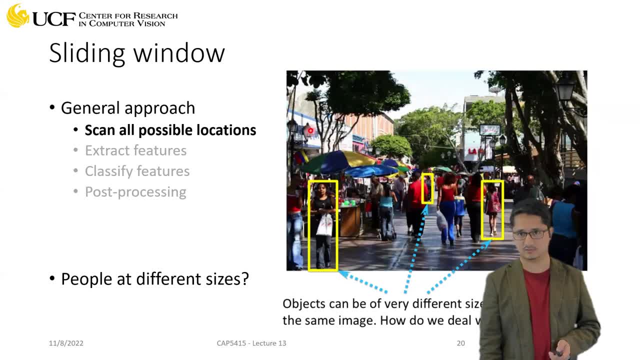 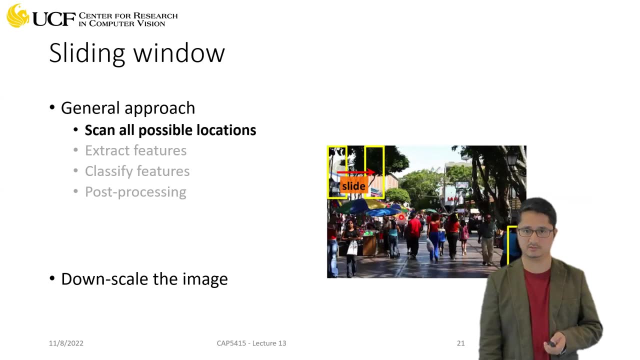 uh, we try to scan the images at different resolutions, okay, so this is just showing that. okay, for, uh, the close by people you have, you have bigger bonding box. you call it your image size. so for the farther away, you need a smaller bonding box, and what you do is you resize. 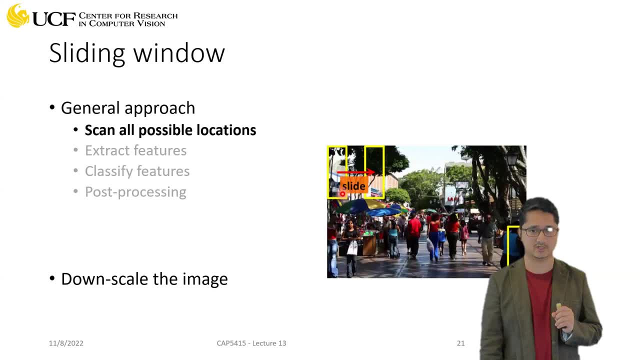 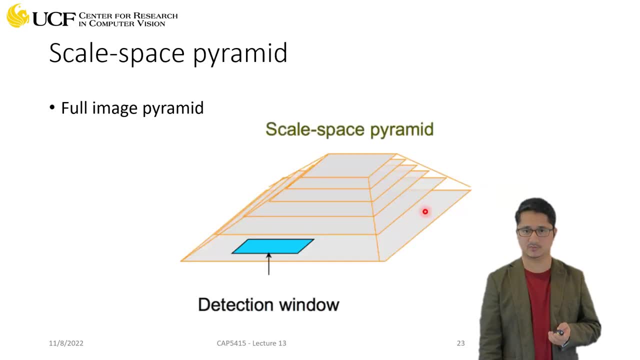 your image, you resize your image, but you keep the size of the bonding box same. you don't change that. okay, you keep reducing and you will create like a scale space pyramid, exactly the way you were doing for shift features. so this is like a bigger resolution and this is your detection window now. 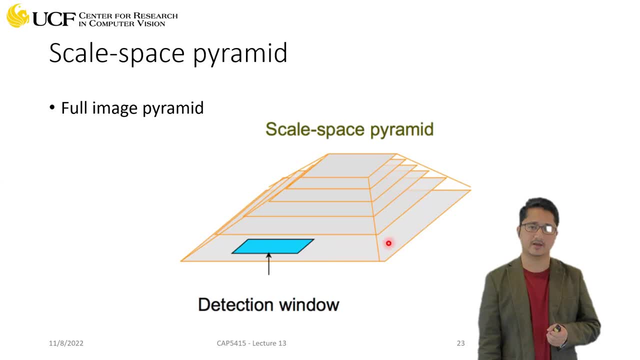 you can see that uh resolution image. you're actually trying to detect the the smallest scale of your object. okay, and the idea is, if you are using this detection window and this is, let's imagine, one particular individual, so that will be like height and width of that individual, right? 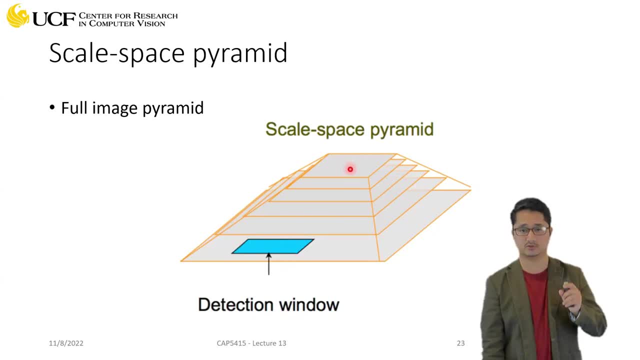 but if you're using the same detection window on this scale, which is on the top, then you can see that the the actual size of that person is much bigger than that. so, although like this is kind of an inverted pyramid, but the scale at which you are detecting- 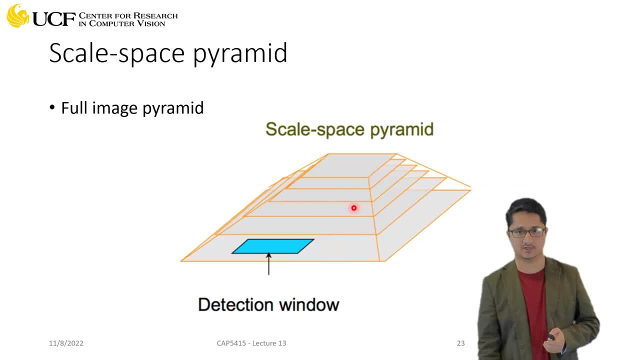 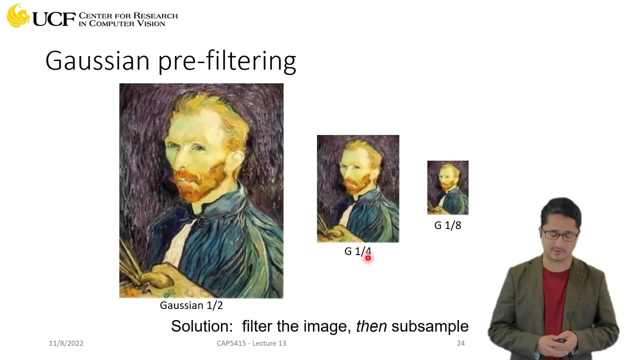 your, uh, your objects. it's actually kind of reversed, okay, so the top one will detect like bigger, uh, bigger scale objects, and the bottom part of the pyramid will detect like smaller scale objects. all right, so one important step while uh, while we do that is, uh, gaussian filtering, and again you have seen this like why, uh, smoothing is. 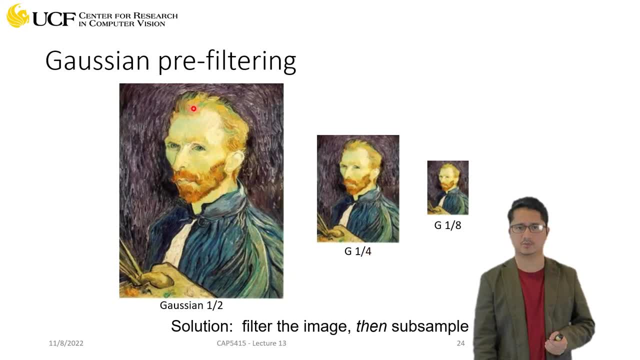 really important. so what we do is we try to do some kind of pre-processing, using uh gaussian filter to smooth out the image, and i will tell you, like the reason, the exact reason why we need to do that. so this is like your image at high resolution and as at each like step of the 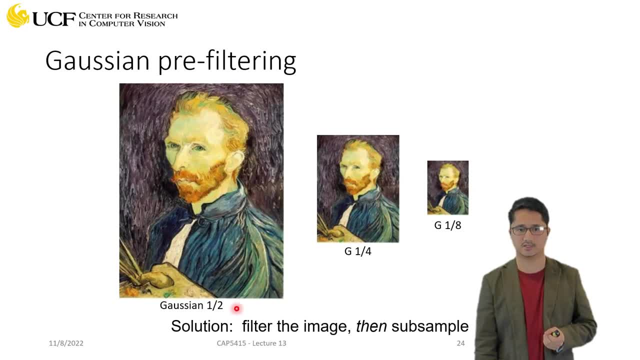 pyramid. you are reducing the resolution. okay, you are going from, let's say, with 600 it will be 300, then 150, so on and so forth. now the question is, when you do that, then again there are different ways to do it, how to go from this image to this. 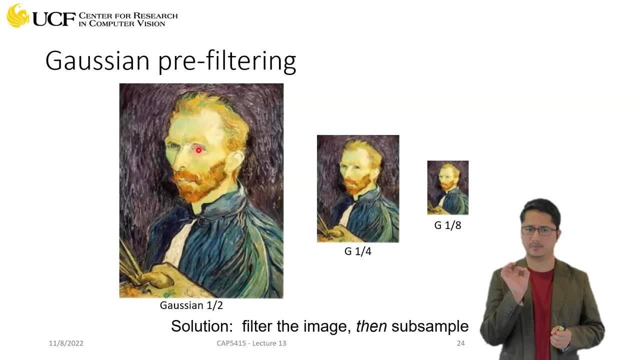 image. one simple way could be: you can just pick like alternating pixels and you skip some of the pixels in between. okay, so that will give you exactly like half resolution. for example, if, uh, the number of columns in this image is 600, then we don't pick all the pixels, we pick like. 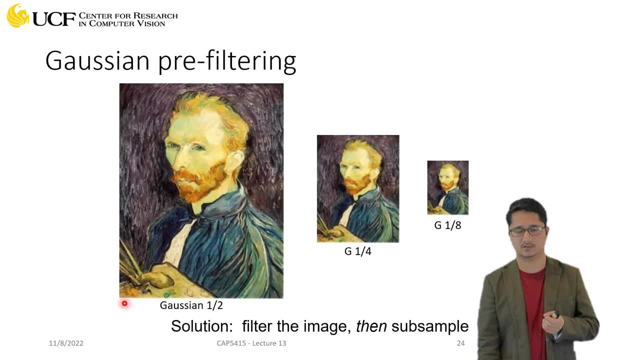 alternating pixels, let's say odd pixels or even pixels, and then you will exactly get 300 pixels and your image will be like just half half resolution and you can keep doing. when you go down now, while you are doing that, what's happening? you're actually omitting those pixels, so you are actually clearly missing. 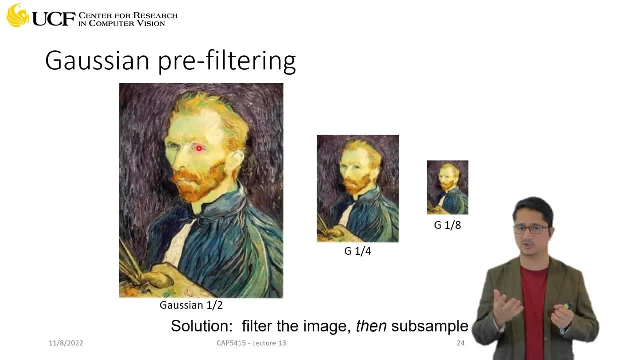 those out right. if some important information is stored in those pixels, it will be gone, and that's why we need caution pre-filtering. what will happen is, if you're doing gaussian smoothing, you know that when you place a gaussian filter at some location, you make use of values from the neighboring pixels. 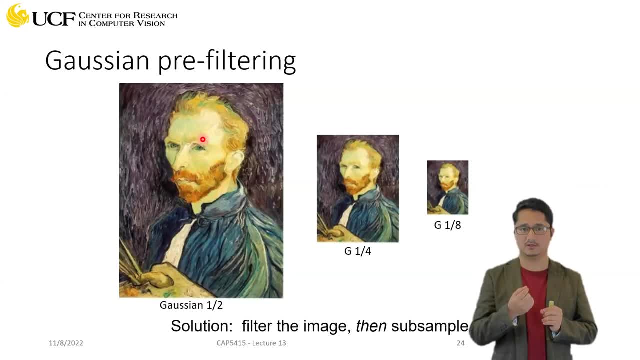 that's how you smoothen your image. and if you do that, then the sub sampling step, where you were actually skipping some pixels, even though you are skipping, but information from that pixel was actually already captured in the pre-filter, the pre-filtering, uh, the pre-filtering step. 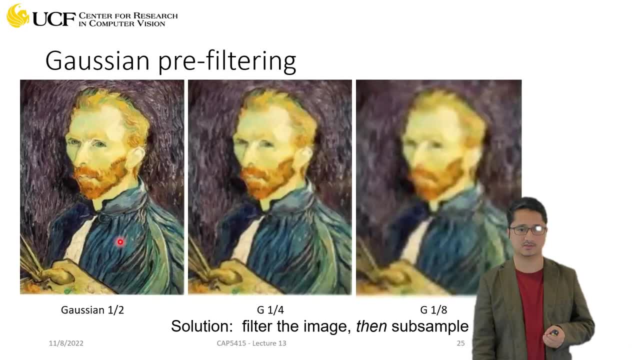 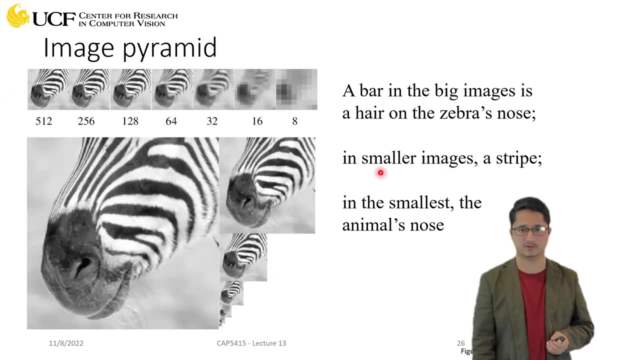 okay. so now this is like something which you will get, because this is high resolution and you keep, you're reducing the resolution after smoothing, so you can see like that's the effect of smoothing, uh, which is fine. but if you try to look at the, uh, the, the local level feature, uh, what you're. 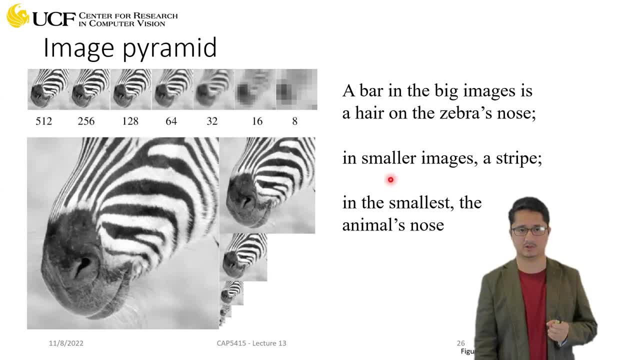 going to get from these, these image pyramids. now, if you look at, uh, this bigger image, right, so it could be like one pixel is actually maybe one stripe here, right, or it might be. it might be reducing and as you reduce the resolution, it could be like one pixel is just representing. 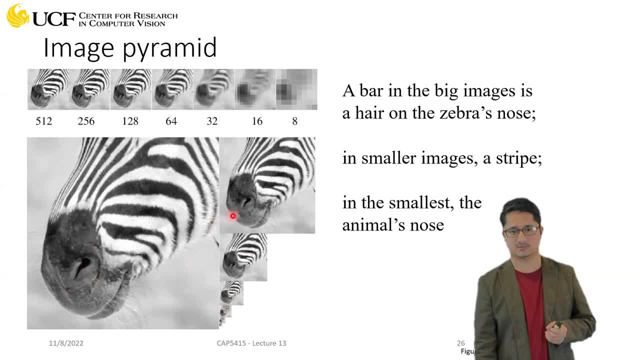 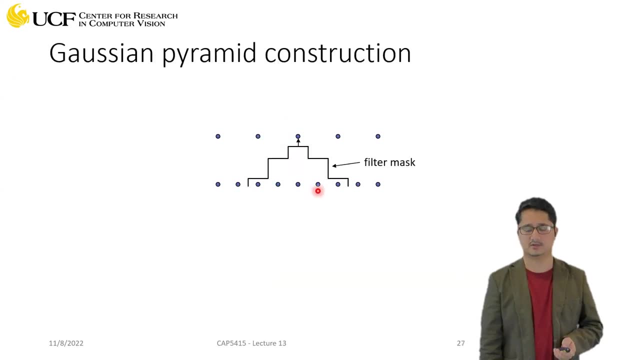 maybe the nose of this zebra. okay, so that's how you're actually controlling the, controlling the scale. so it's going like from five, one, two, all the way to eight, so you have like six, seven different scales. okay, so the way this uh pyramid construction works, is you? so? these are just showing you. 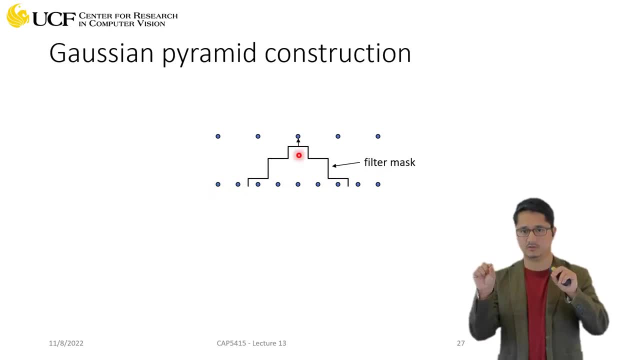 pixels and or even though this is like just one row, but you will have a full two-dimensional space for that. okay, so just consider like one row of your image, which will be consecutive pixels. so, and this is just showing one dimension, so you will use your gaussian filter, which is something 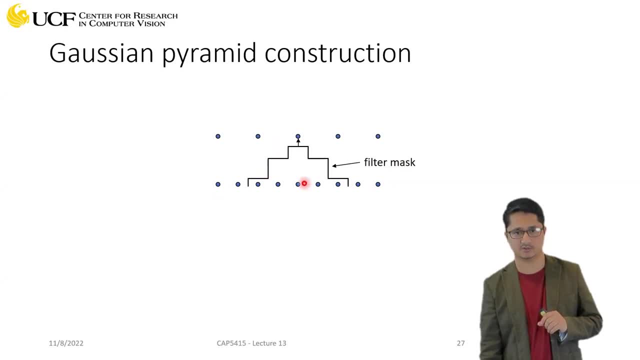 like this: right, you will pay more attention to the center pixel and less attention to the nearby pixels, and then that's going to give you this pixel. so it's kind of average of all these. so this is your first like one scale of a gaussian pyramid and this is the next level. so in this 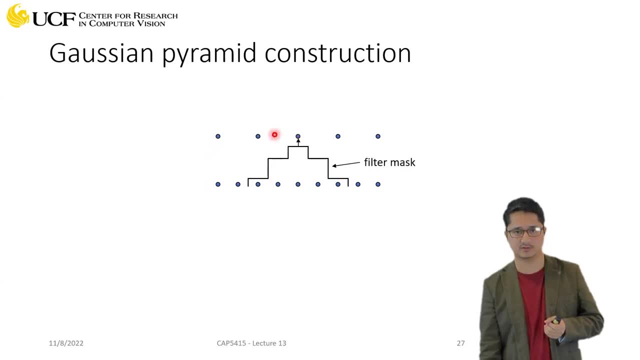 case, you can see that whatever value you're getting for this one, you just skip that. so you are just alternating between pixel values, so you are reducing the resolution. so you perform filtering, you perform sub sampling, skip those pixels and you keep doing that again. if you do like a gaussian filtering of this, again you are considering all these. 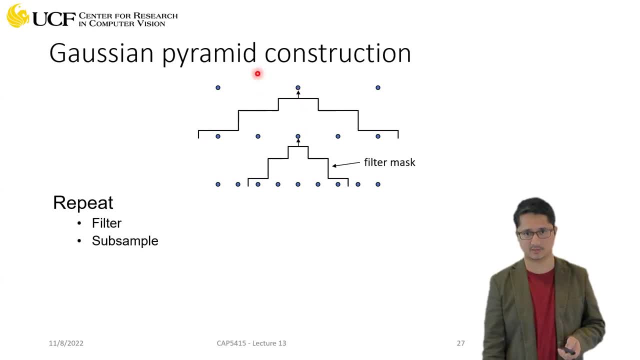 pixel values to compute this one. but again, you skip in between. okay, it's just making sure that if some pixels have, uh, important or salient features, they are not skipped over and again. this is one dimension. you can easily generalize to two dimensional space as well. now, if you think, 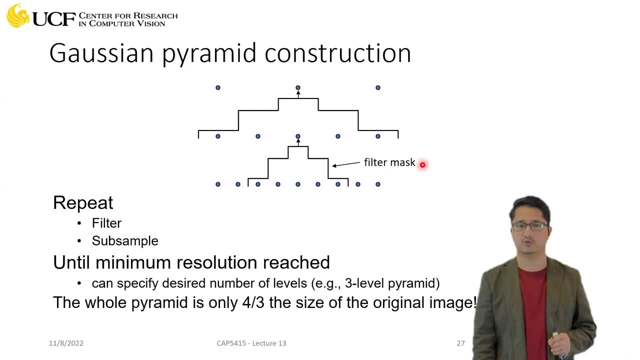 about this, uh, the total amount of memory you require to store like this, uh gaussian pyramid, it's not that huge, even though if you have like a lot of layers, let's say three level or four level it, it won't be a lot, because let's say, if this is uh saving n pixels, this is just going to be n by. 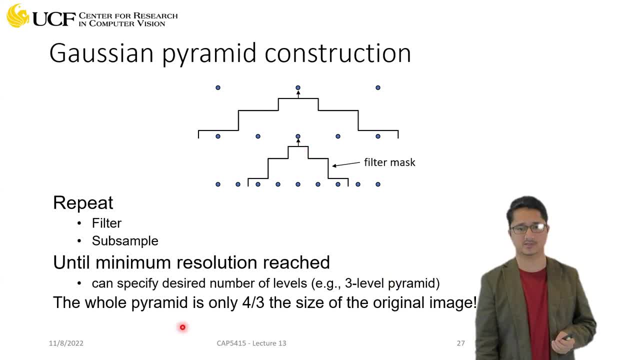 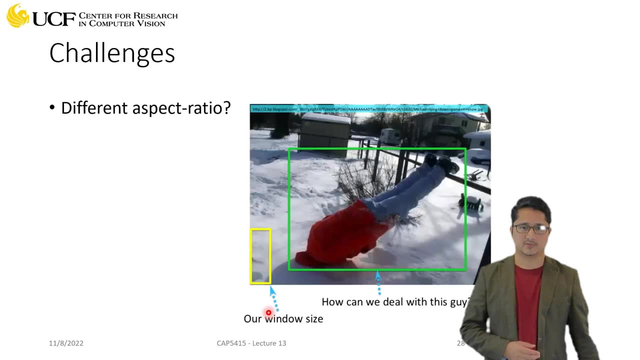 two pixels. okay. so for a three level you will see like it's just like four by three of the size of the original image. so in terms of memory consumption it's not increasing your memory consumption by a lot. definitely it's never going to go to like 2x okay. so now the issue with like 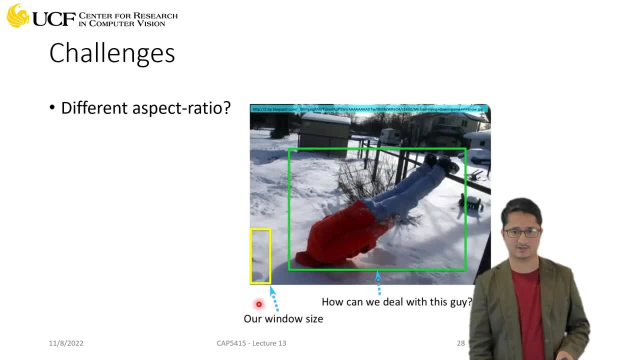 that uh kind of approach will be, since we are looking at this specific aspect ratio. you might have individuals in your images, something like this: okay, there will be all the way all all sort of variations out there in real world. so, whatever you do, but if you have this kind of window, it doesn't matter how many scales you use. 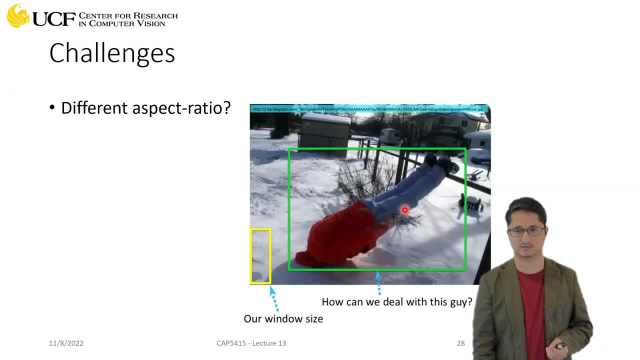 you are always going to miss these kind of detections, okay, but again that's just one challenge. and of course you can try to do maybe different aspect ratios, but again that will just increase, like the computational complexity, and whatever you want to do, you can do it. you do, uh, with one set of aspect ratio. you will have to repeat that with a lot of other aspect. 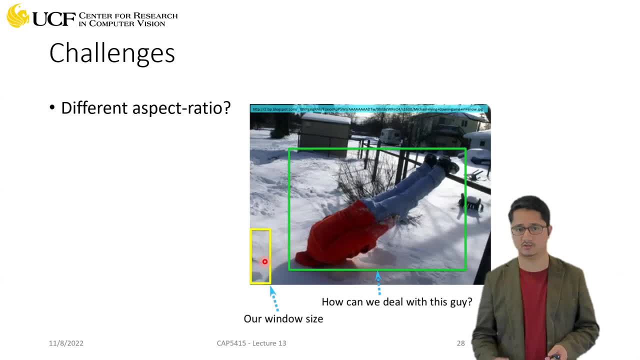 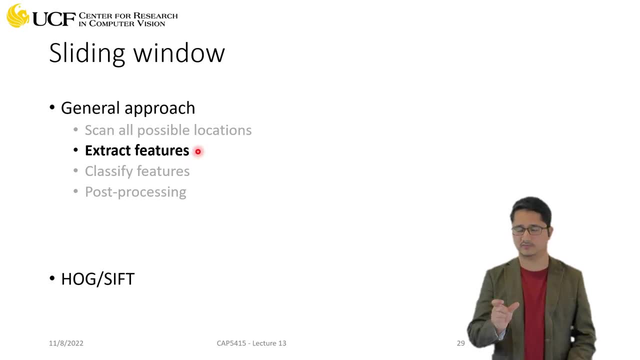 ratios and we will see later on, like in in the actual cn algorithm, how this is being addressed. now, once that is done, you just extract features from that block, as i said earlier, and it's up to you like what kind of features you want to use. it could be classical features, it. 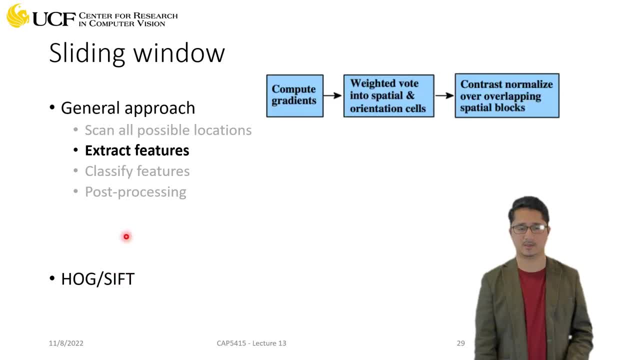 could be your deep learning features. everything is fine. now, here's the, here's the trick. here like: so it's fine, you can extract features, but how will you classify, right? so the way it works is, as you know, that if you have to do detection, you need uh labels for annotations, for that right. 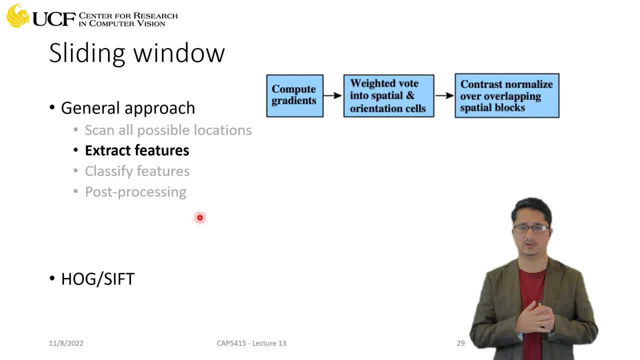 so for training samples, you should know like what exactly that bonding works will look like. so what you do is, during training again, you try to scan like those possible locations and you will. you will then have like some patches as positives and some patches as negative, because some patches will match the ground truth and some patches will not. 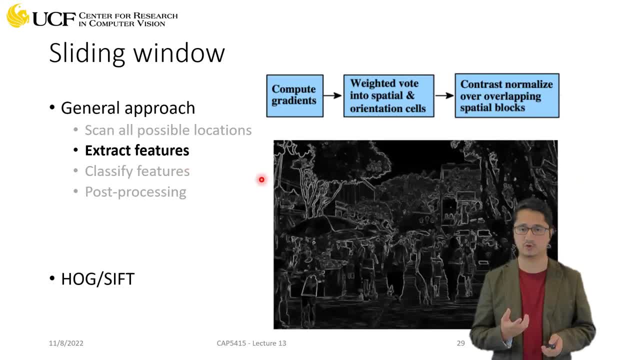 so then what you can do is you can just collect those uh bonding boxes and create like a training set where you would have a positive class where person are present, a negative class where person not are not present, and you can just train a classifier. it could be a simple cnn classifier. 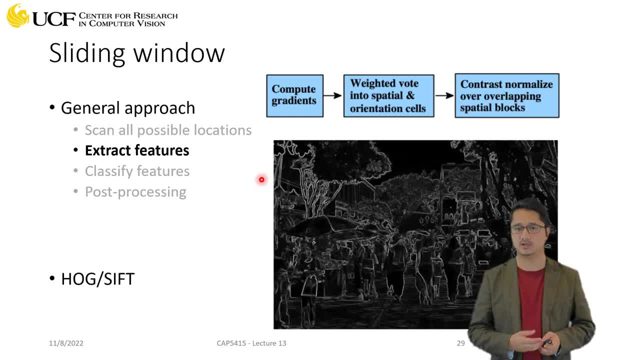 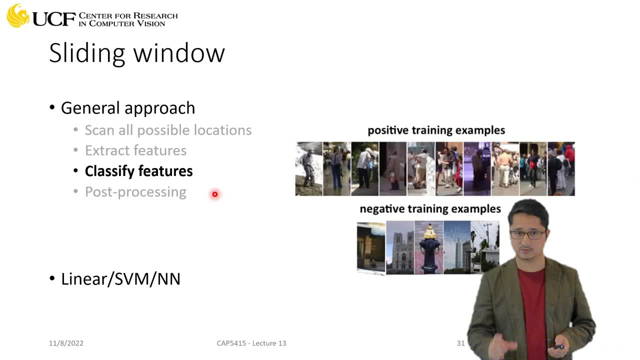 it could be svm classifier, because in this case you have features. and once you have that trained classifier, then you can use that train classifier during testing time. and during testing time again, you take the same window, keep scanning on the images and then that classifier will tell you whether person is. 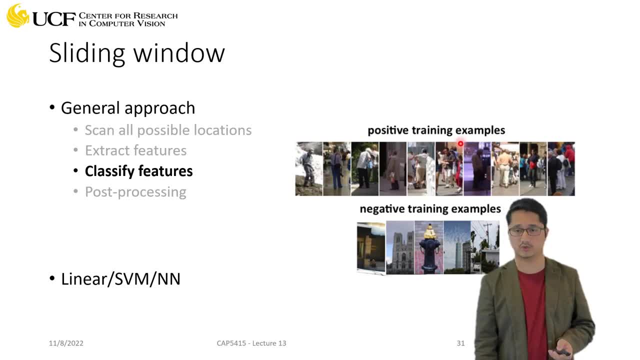 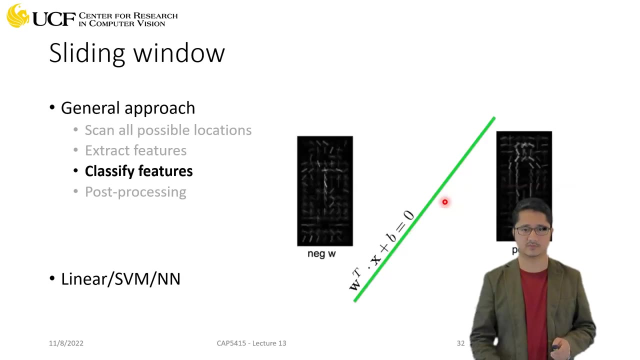 present at that location or not? okay, so this is just showing some sample uh examples which will be used for training. so all these are like positive cases because you have individuals present, and all these are negative examples. again, you are extracting these samples from your annotations, okay, so then you simply 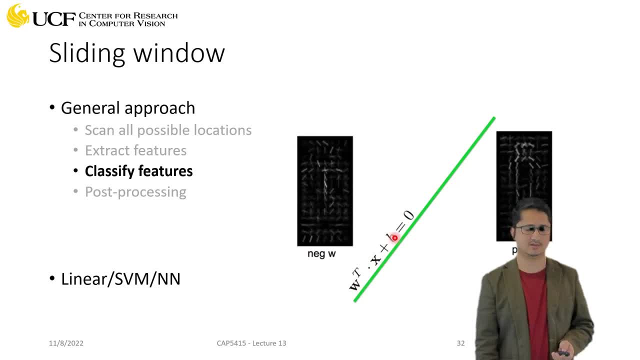 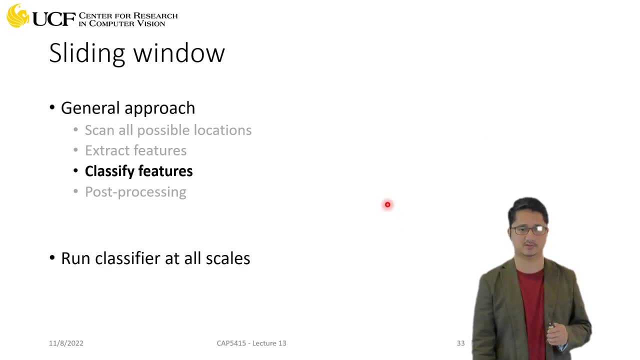 train, like maybe a linear classifier, something like this: it's up to you, like what kind of classifier you want to train, and we have seen, like uh training classifier, i think, two different variations at least. okay, so once that is done, we, uh, we try to use that classifier to make predictions. 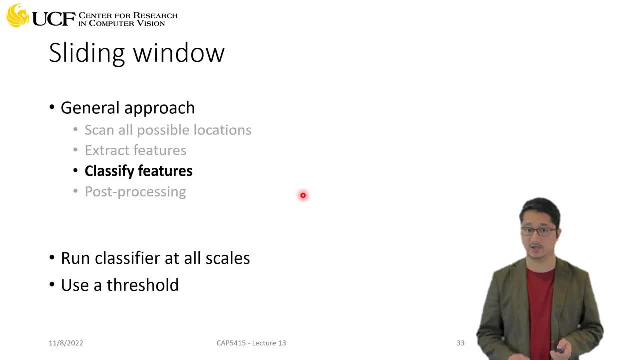 whether a person is present or not. and again, we do that at multiple scales. and of course, for your, for preparing your training data, again you will do that at multiple scales itself. right, so that that will help. so you, you'll have to use some kind of threshold to say that, okay. 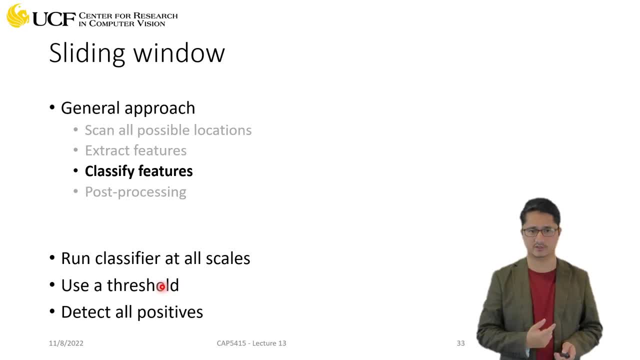 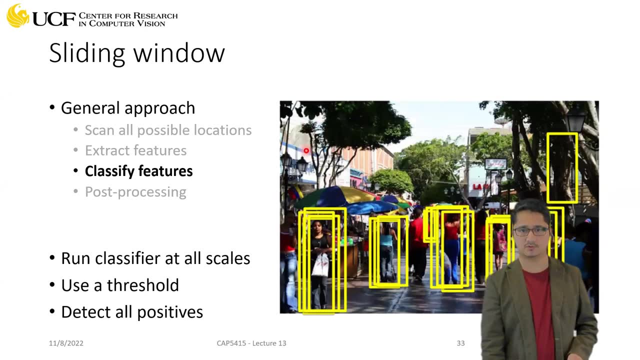 object is present or not. again, that's part of a classifier. you know, know all that and this is, let's say, some sample result. you have this image. you again scan all the pos, all the possible uh locations, and then you try to classify all those possible locations and then your algorithm might 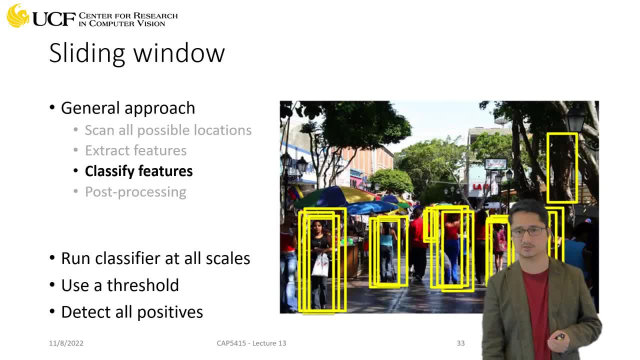 have said: okay, at this location, person is present. at this location, person is present and that confidence level might be higher than the threshold. okay, so remember, you need a threshold for a classifier and if it's a binary classifier you can say that, okay, point uh, five and above it's. 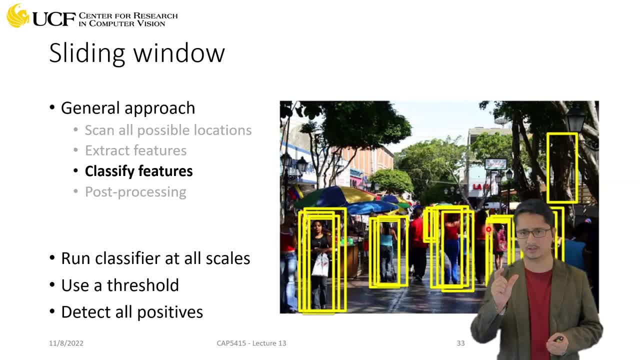 a positive case, point five and below it's negative case. so it's up to you- and again that's like a parameter, you, you have to decide. and let's say, all these bonding boxes were detected, directed as positive. yeah, you can see like one issue, you can clearly see like at one location you have. 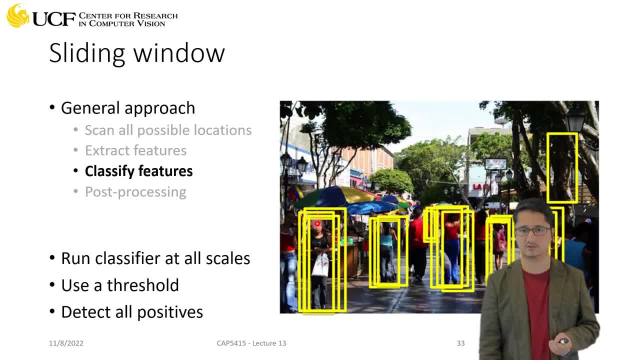 multiple bonding boxes, which in which, in a way, is right because all these are correct, right, you have this individual present here. but then the question is: do we really need that many bonding boxes? in this sense, the algorithm is saying: okay, one, two, three, four, four different individuals are. 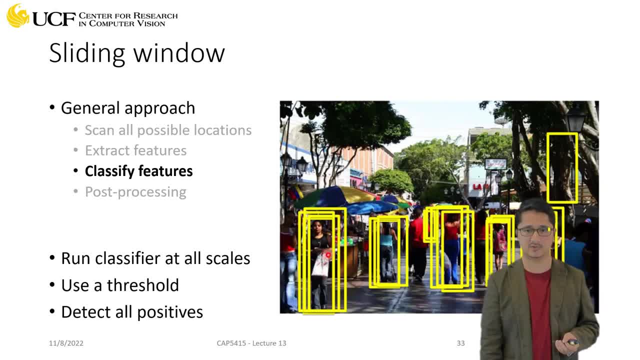 present. but that's not true. we can only see one and again. the other interesting aspect: you can see like you have some smaller bonding boxes as well, which means that you were able to take care of that scale aspect because you were trying patches at different resolutions. okay, so now. 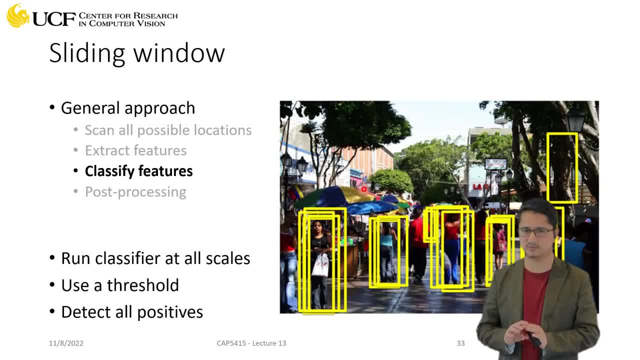 so that's fine. so that's like a initial step. you have these predictions, which is kind of already giving you results. but now we need to improve on this, and that's called post-processing. so we need to get rid of, like these additional boxes. okay, so let's see how we 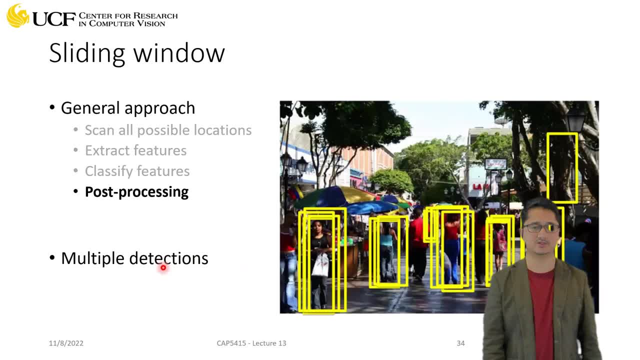 can do that. so, as i said, you have multiple detections, uh, and that that's not good. so what we use? we use non-maximal suppression and we have seen this algorithm before, if you remember, like your edge detection algorithms. that's exactly what we were doing there. so the high level concept. 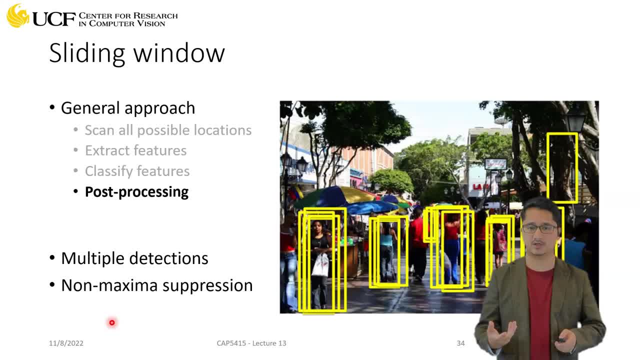 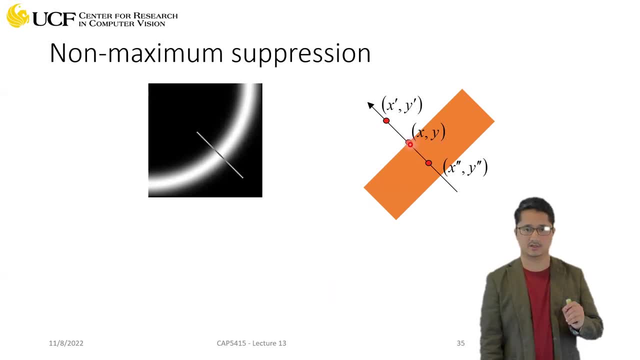 is not going to change. okay, it will remain the same. it's just a different kind of application. so, if you remember, like from edge detection algorithms, uh, what we're trying to do is at any given location or any pixel location. we were looking at the neighboring pixels. 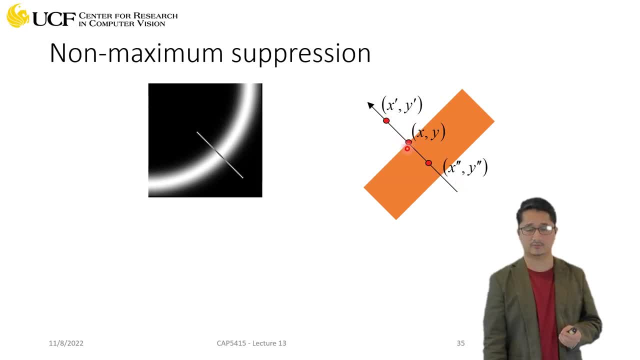 right in the direction of the orientation. and if the magnitude of this edge being detected is greater than the neighbors, we say that this is an edge. but if it's not, uh, greater than these two, we say this is not an edge. so it's kind of you're. 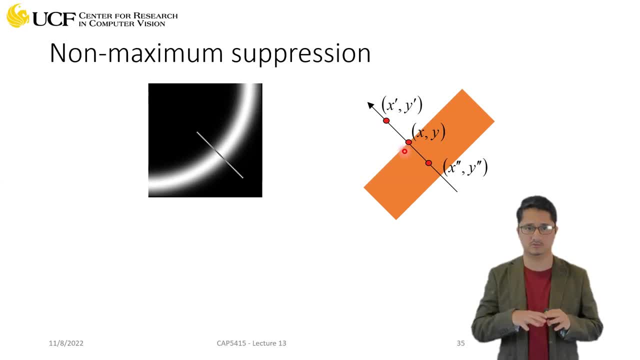 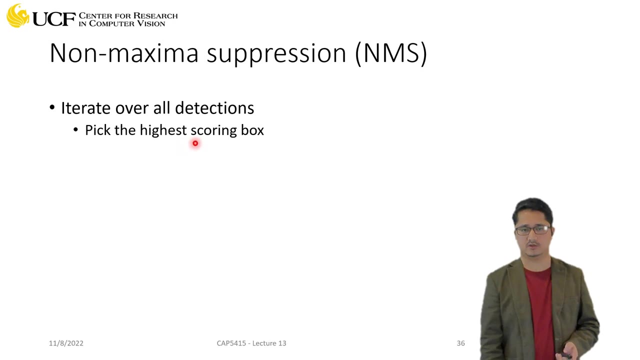 suppressing. if it's not like dominant in the neighborhood, okay, so that's the name, like non-maximum suppression. if it's non-maximum, we suppress it. so the idea remains the same, but what we do here is it's like slightly modified algorithm. so whatever detections you have for any given image, it will be a long list right, because you might have. 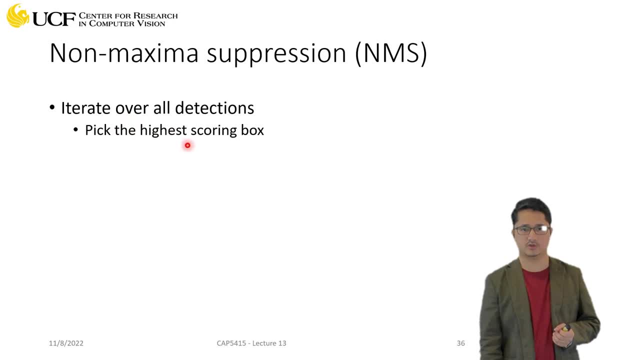 multiple objects present. now, what you do is you first of all sort, like all the detections based on the confidence score. okay, so what you do is you go to the bonding box, which is like your, your model is actually very confident. it's saying like 100. this is a person. you start with that. now what? 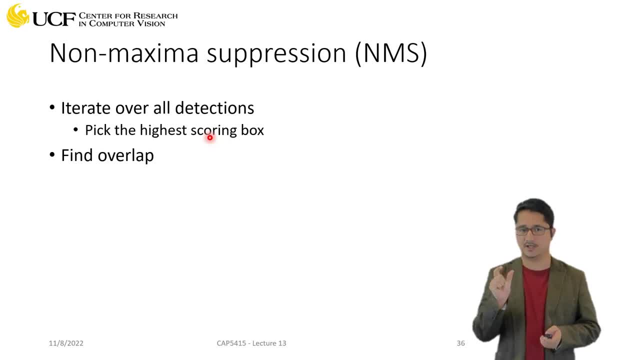 you do is you take that bonding box and compute the overlap of that bonding box with all the other detections, okay, and the kind of overlap you will compute. it's called intersection over union and again, this is a very important term i think you're using for nms. that's fine, but i think if you're solving 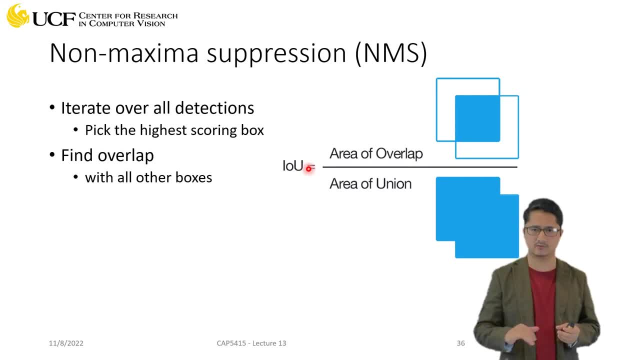 detection problem, like whether you do evaluation, whether you like do some kind of uh loss computation, you will see like different variations of this intersection of your over union. so try to understand, like, what this does. so, first of all, you have two different detections. okay, so there are two. 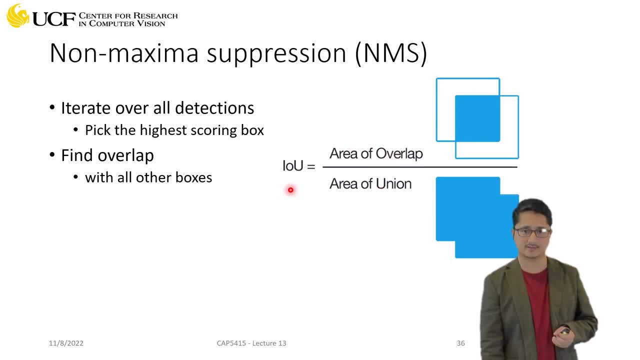 of them. so that's numerator and denominator. so in the numerator, as the name says, intersection over union, right? so in the numerator you will have intersection and in the denominator you have union. so intersection means what part of these two bonding boxes is common, and in this case you can. 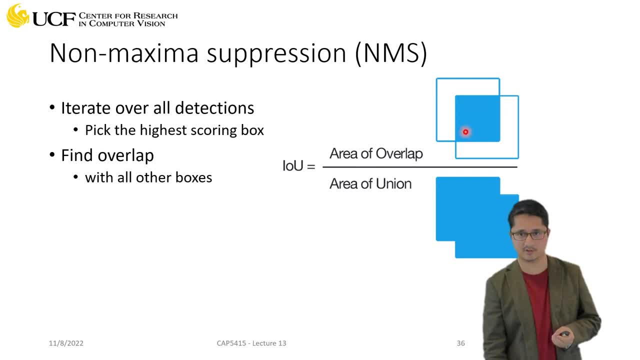 see, like this blue region over here, that's the common part, right? so we just found, uh, we find this area, whatever this area is, we put that in the numerator. and union is we just combine, like both the detections find, like the area of this overlap or not overlap, just like the the union of these two bonding boxes. 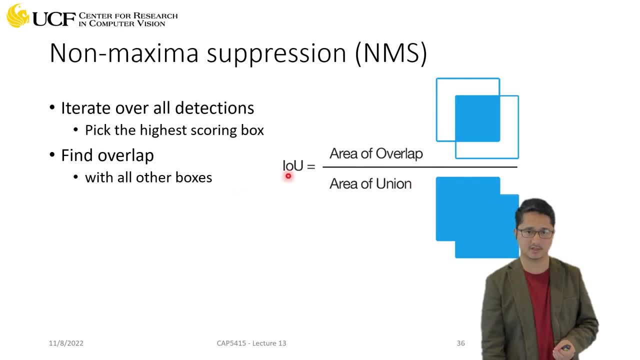 just blue color over here and we put that in the denominator. so this intersection over union will tell you, like what's the overlap between two different bonding boxes. okay, so you, you, you do that for uh, all the uh bonding boxes you have. you start with the highest one and then what you 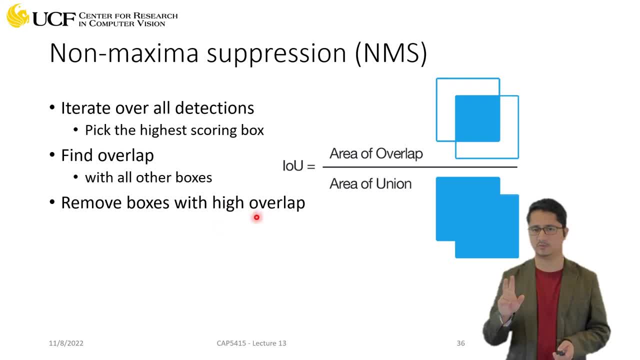 do is if you find like there is like a high overlap between two different bonding boxes, you will keep like the highest scoring bonding boxes, but all the others you will just get rid of them, we just remove them. you say that it's not detection anymore. okay, now one one trick here: 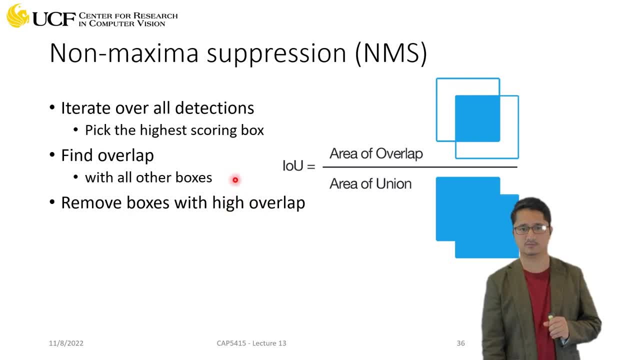 so the trick is it's saying like high overlap. now the question is, how do you define high overlap? and that's kind of arguable, and if you change a lot, like your performance a lot, and so again, this is, like you can say, a parameter, and even when we try to evaluate these object. 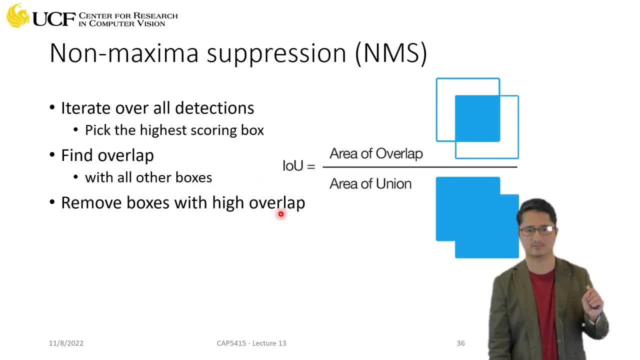 later we will see. we make use of this uh threshold as like one parameter, so we try to compute the performance of the algorithm at different uh thresholds. okay, so this part is actually important. we will revisit this later, but for now you can say that, okay, we have some kind of 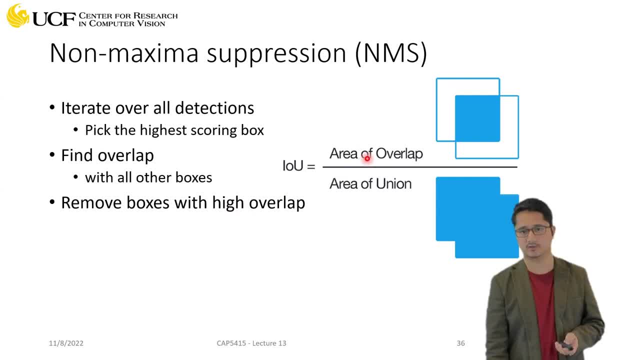 threshold. if iou is, so this is going to be like between zero and one right, so the best score you can get is one, which means that it's a perfect overlap, because what will happen is your intersection be the area of the square and your union is also going to be the intersection of that square. 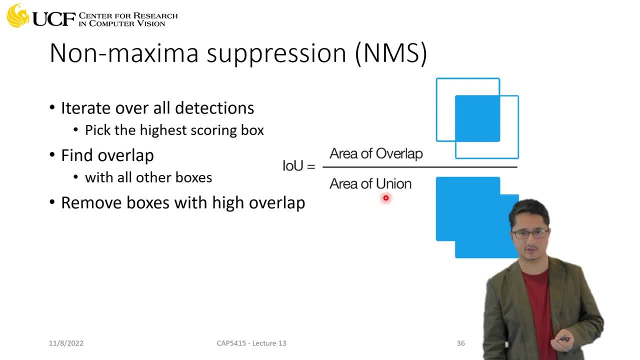 because it's perfectly overlap. they are on top of each other. because the maximum score is one, the minimum is zero when there is no overlap at all. so union will be a big number. numeratory will have completely zero. so then you can set a threshold. let's say 0.5, and say that okay if it's greater. 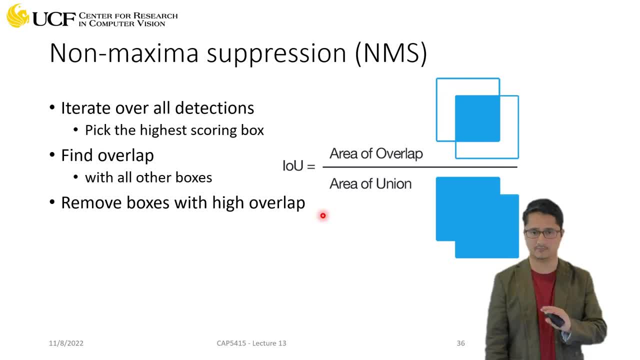 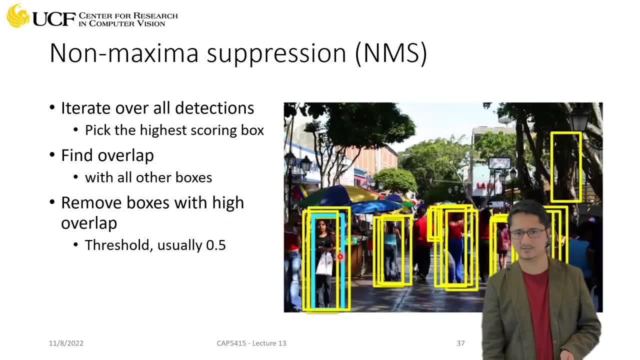 than 0.5. it's an overlap. if it's less than 0.5, you will keep. keep both of the bonding boxes, okay? usually it's 0.5. now let's try to understand with a simple example over here. now this blue bonding box over here. 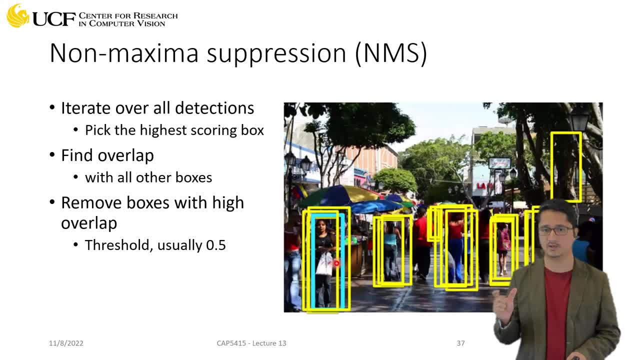 let's say that was the bonding box which your model was saying: with the highest probability this is a person. so we start with that and we compute the intersection over union of this bonding box with all the other bonding boxes and clearly, visually you can, if you inspect this, you 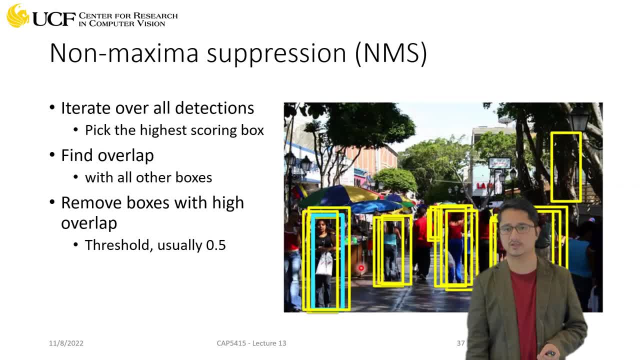 can see that all these bonding boxes, boxes on the right, literally there is no overlap at all, so you will still keep those. but now if you look at, uh, these bonding boxes which are, uh, in the neighborhood, so some of these will have to go away and again, that will depend on whether the intersection over union is greater than 0.5 or not.